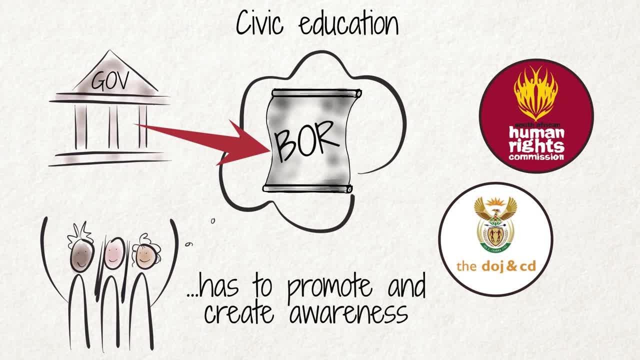 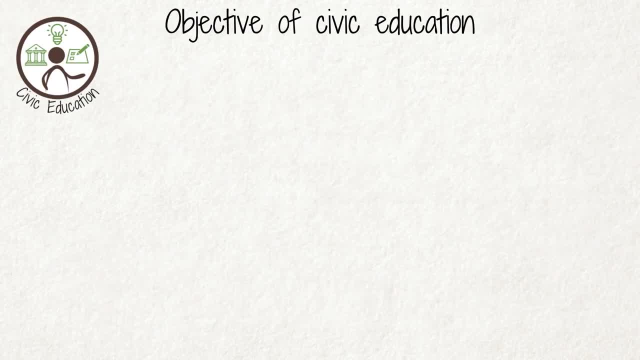 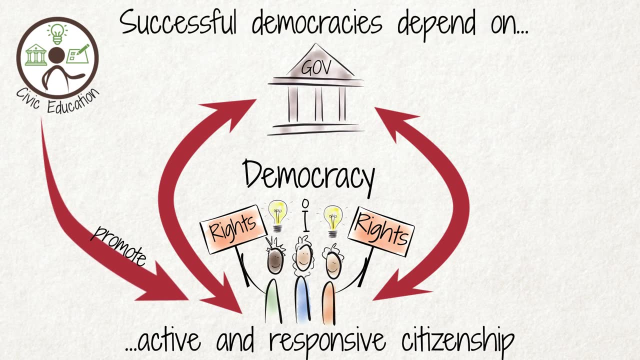 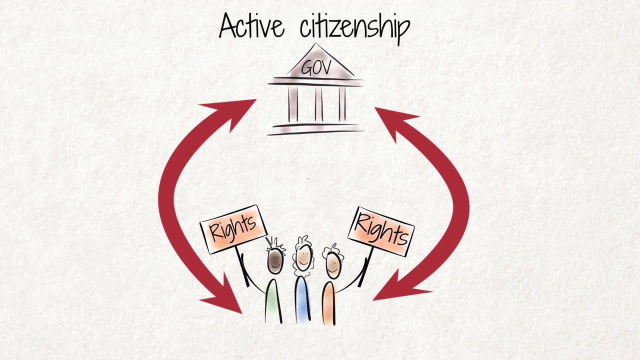 The Department of Justice and the Human Rights Commission are some of the state institutions which have to promote this type of education. The overall objective of civic education is to promote active and responsible citizenship. This means that democracies critically depend on active citizens- People like you and me, upholding and claiming our rights. 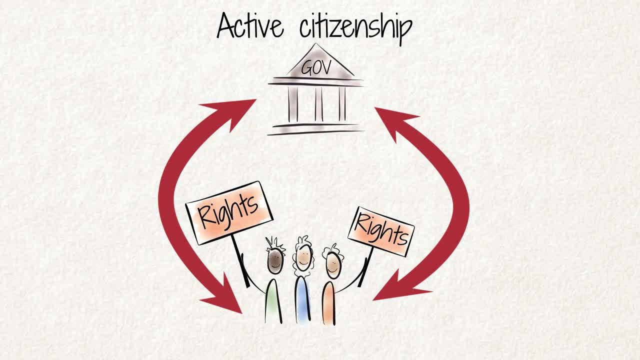 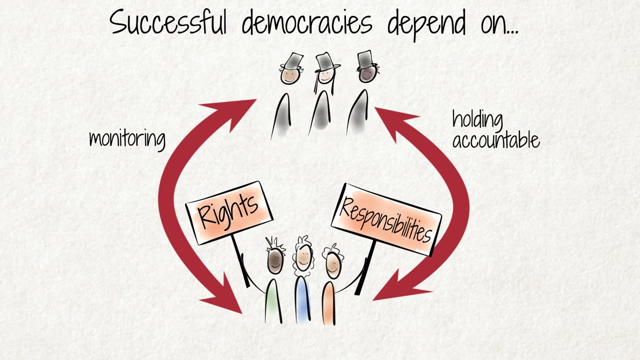 But active citizenship is not only about having rights. It is also about living up to our democratic responsibilities. For a democracy to function, it is the responsibility of people to monitor the performance of our government and hold political leaders accountable to fulfill their promises and to serve the people. 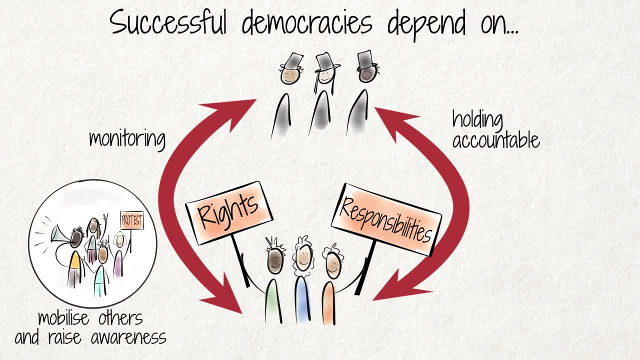 If we see that things are going wrong, then we need to stay focused right. If we see that things are going wrong, then we need to stay focused right wrong. we can mobilise others in our community to raise awareness, change policies or ensure. 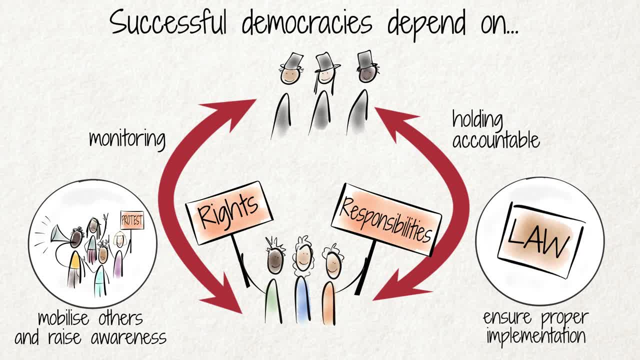 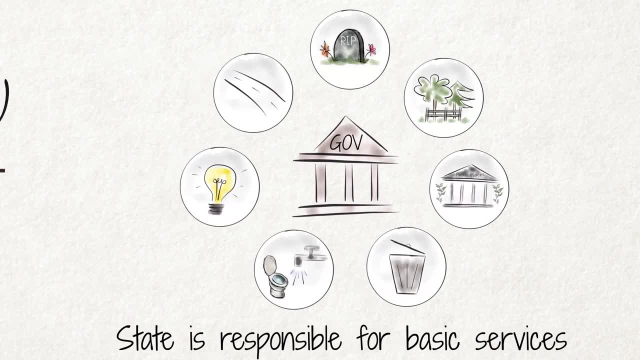 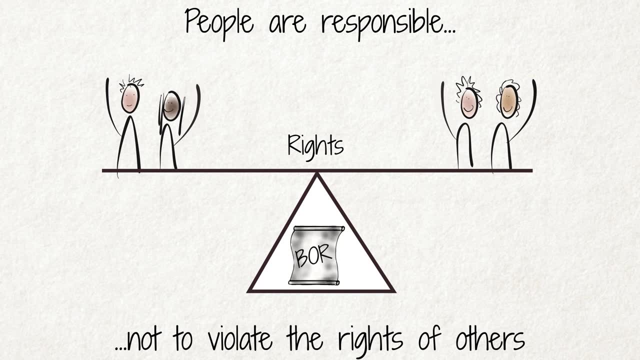 that proper implementation of policies and the law occurs as it should. While the state is responsible for providing basic services, it is up to the people not to violate the rights of others. Let me give you an example. An essential political right in a democracy is the right to vote. 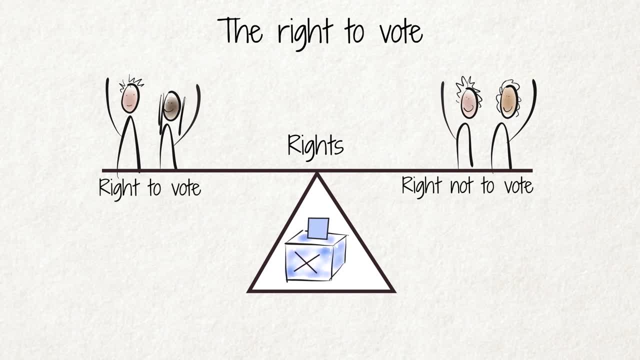 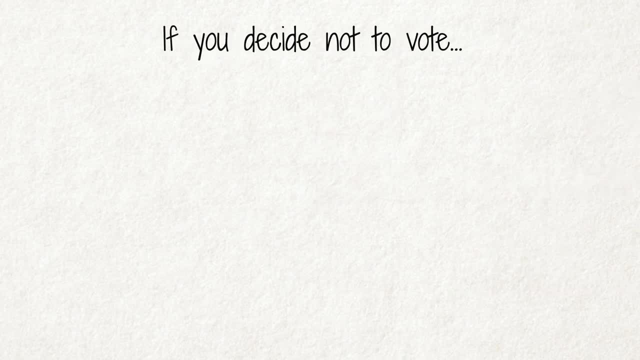 You are not obligated to vote and you are entitled not to vote Should you decide not to vote. that does not mean that you lose any other rights. However, it means that you are reducing the total number of the voting population. If only a small proportion of voters vote in an election, this reduces the quality of 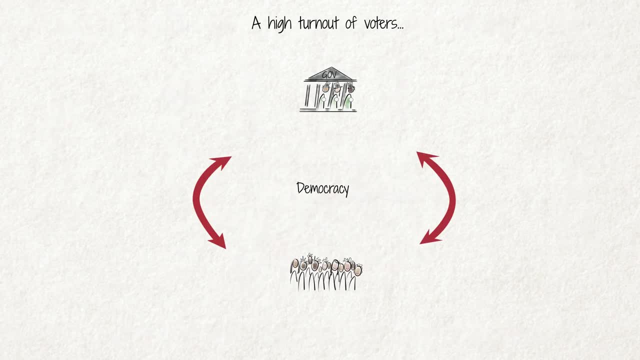 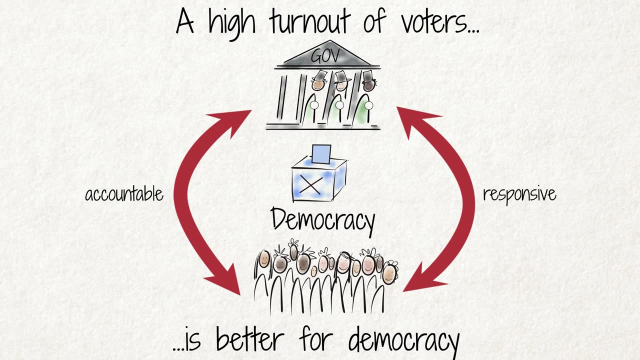 its democracy. A high turnout of voters in elections is better for democracy because it means our elected leaders have more power, More of an incentive to be responsive and accountable to ordinary people. We explain the right to vote in more detail in the video. Why Should You Vote? 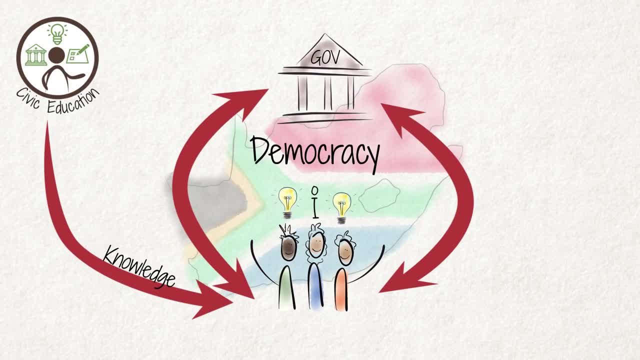 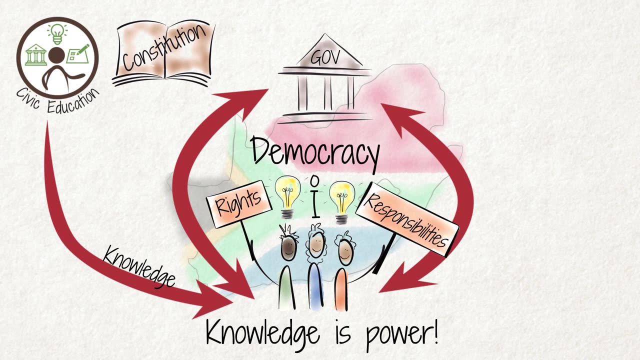 Civic education is about knowledge- Knowledge of what democracy means and how it functions, in line with the South African Constitution. And this knowledge is power. If we are aware of the power we hold, then we can use it to our collective benefit. To use another example, if you know about your constitutional right to access to health,